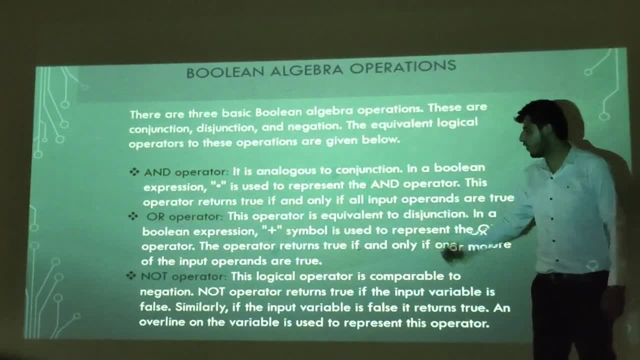 First is AND operator, second is OR operator and third is NOT operator. So what is AND operator? AND operator is analogous to conjunction And it uses dot address symbol, which is also used in multiplication. And OR operator. the operator is equivalent to D. 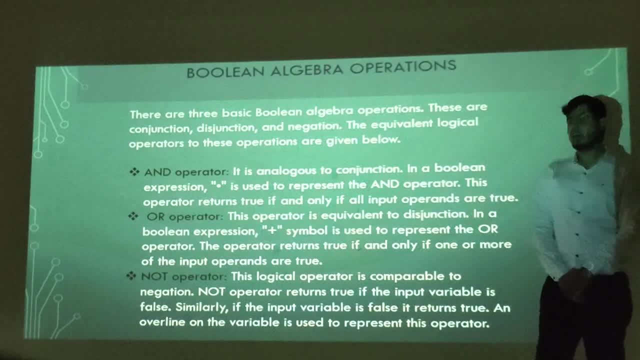 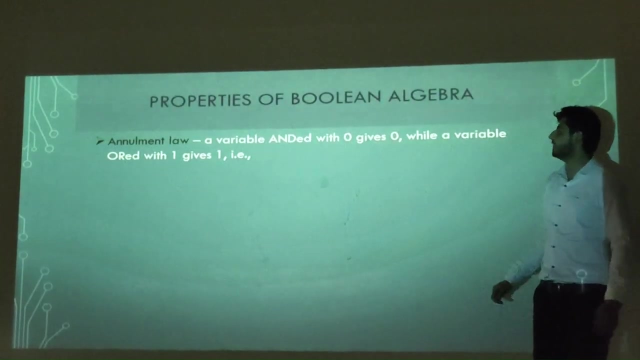 It is junction and it uses plus operation and binaries, Then NOT operator, NOT operator is an operator which do the inverse of the output. So the next topic is properties of Boolean algebra. So what are the properties of Boolean algebra? First is analogous count. 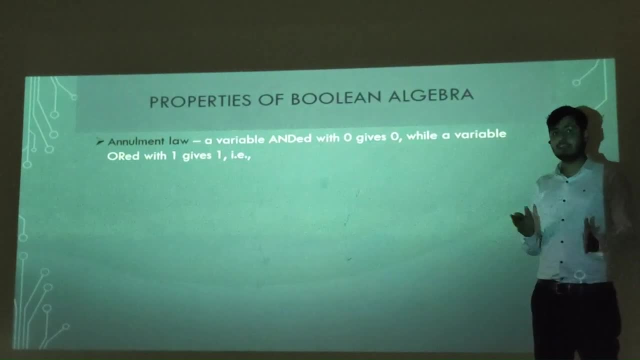 If a variable is added with 0,, it gives 0. While a variable is ORed with 1,, it gives 1.. As you can see here, OR is equal to 0 and AND is equal to 1.. Next topic is identity law. 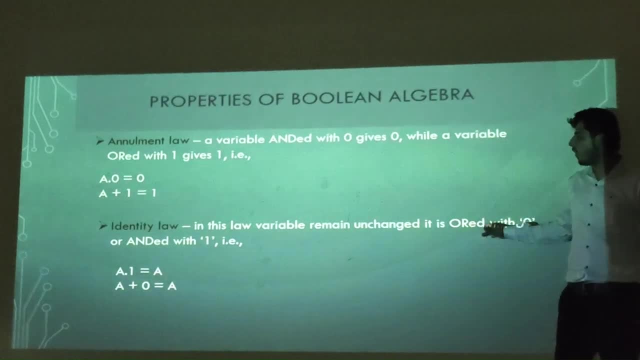 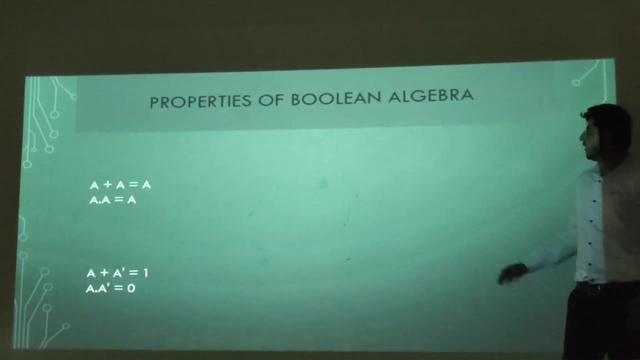 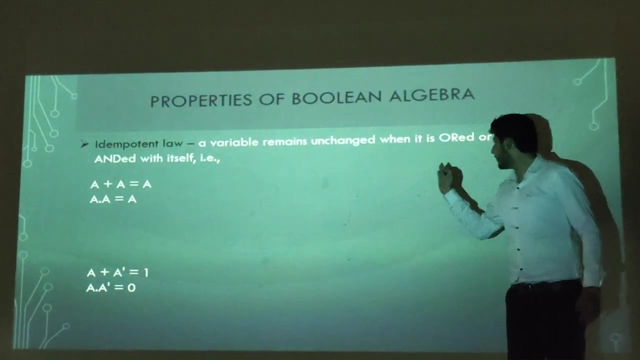 In this law, when a variable remains unchanged, it is ORed or ended with 1.. So, as you can see here, AND is equal to 1 and AND is equal to 8.. Next topic is identity model law. So this law is set when a variable remains unchanged, when it is ORed or ended with itself. 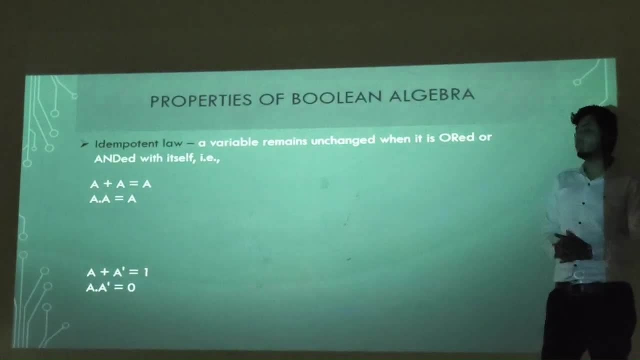 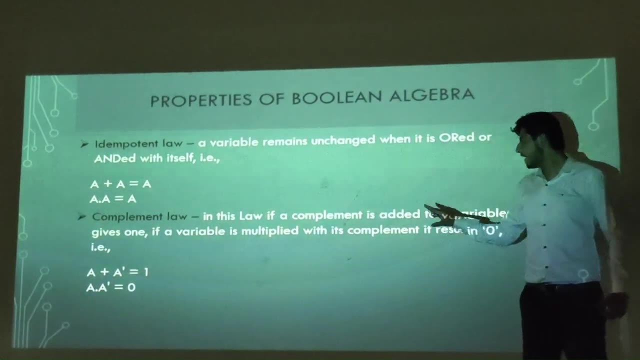 As you can see here, AND is equal to 8 and AND is also equal to 8.. So next topic is ultimate law. In this law, if a complement is added to a variable, it gives 1.. If a variable is multiplied when it is complemented, then it results in 0.. 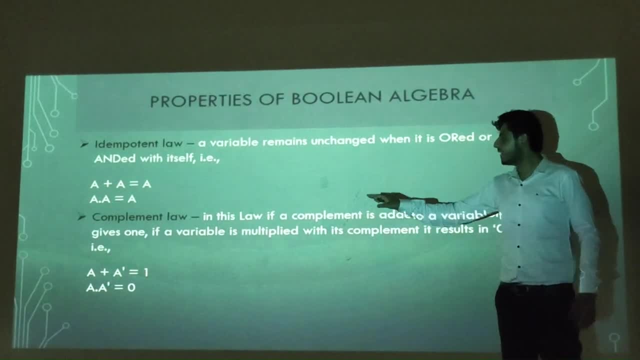 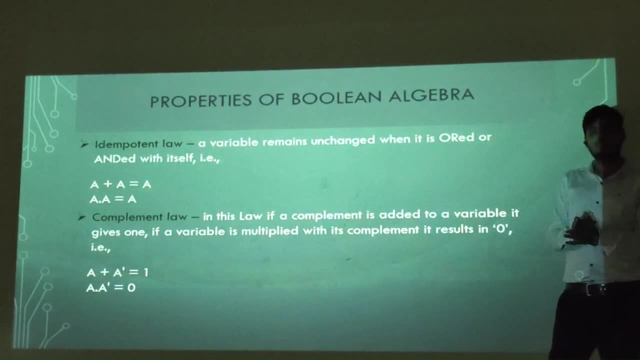 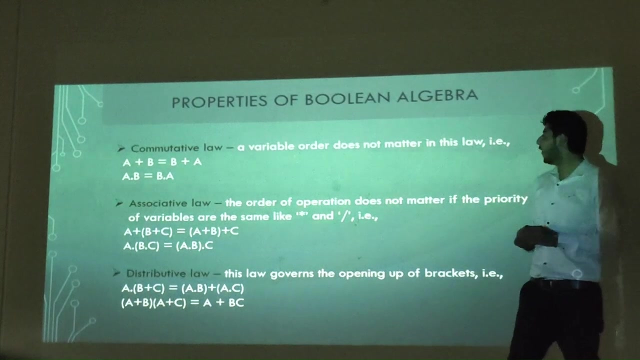 It means that if you add A plus A complement, then it gives 1.. And if you multiply the complement with a variable, A dot A complement, then it gives 0.. Next property is: So what is community law? A variable order does not matter in this law. 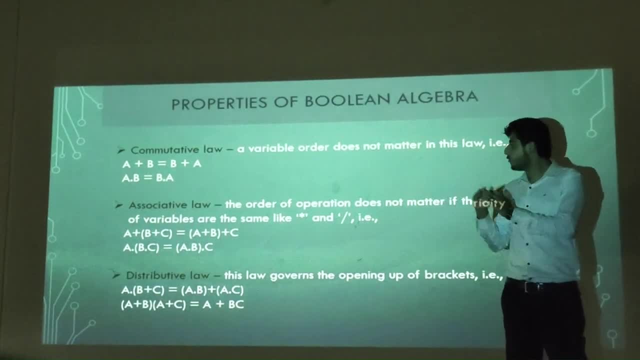 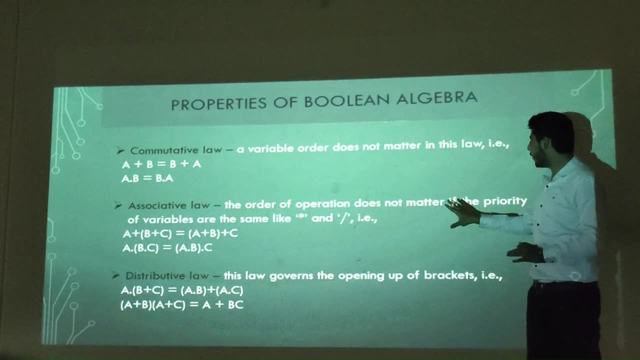 That is, it states that if A plus B will equal to B plus A and equal to A dot B, then it equals to B dot. Next law is associating law. In this law the order of the operation does not matter if the priority of variables are same, like multiplying, divided. 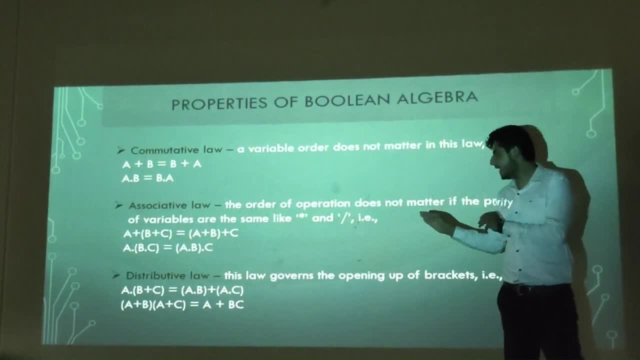 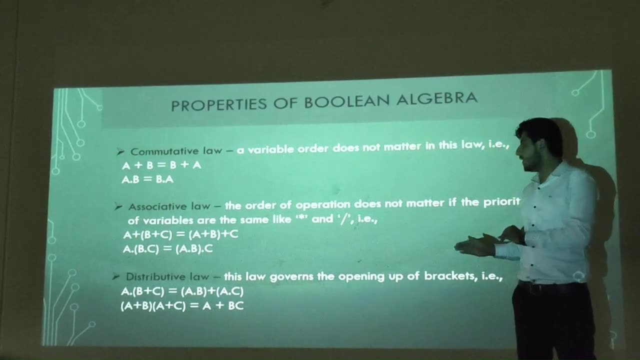 As you can see here, A plus B plus C equals to A plus B plus C, And A dot B dot C equals to A dot B dot C, And A dot B dot C equals to A dot B dot C. So it is distributive law. 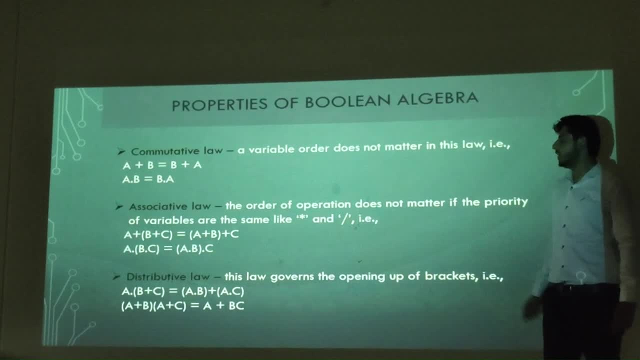 This law covers the operating of the bracket, Which states that if you do A dot B plus C, which equals to A dot B plus A dot C. And another example is also there: A plus B dot A plus C, which equals A plus B dot C. 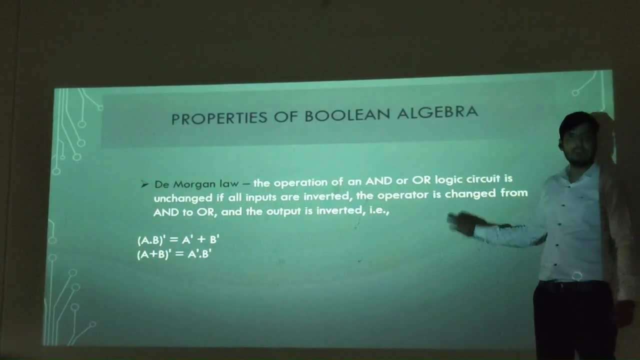 So next property is demodal law. This is very important law in our syllabus. The operation of an AND or allergic circuit is uncheating If all inputs are inverted And the operator is changed from AND to ALL and the output is inverted. 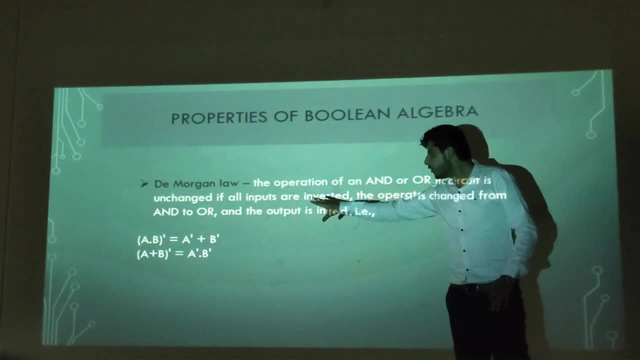 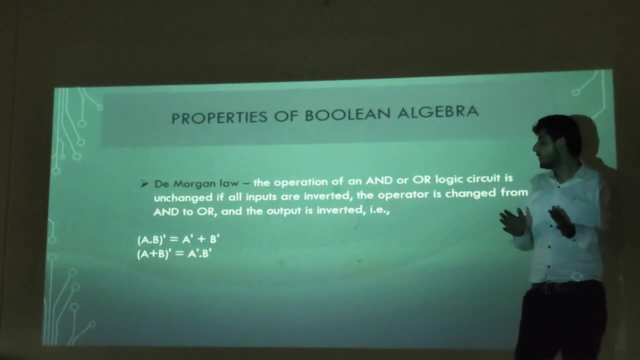 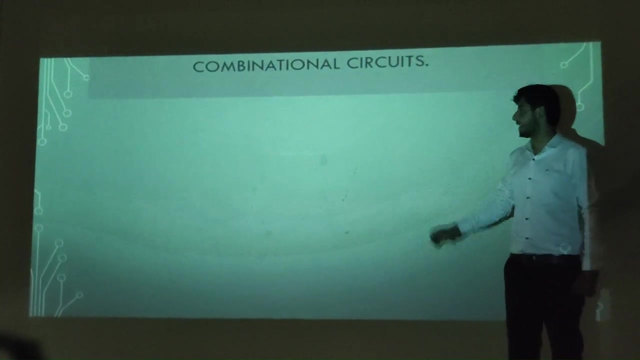 This is very complicated. So I have simple A dot, B whole complement, which equals A complement plus B complement, And A plus B whole complement, which equals A complement plus B complement. So next topic is combinational circuits. So what are combinational circuits? 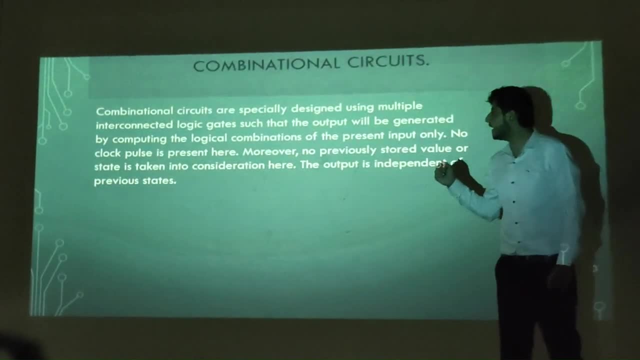 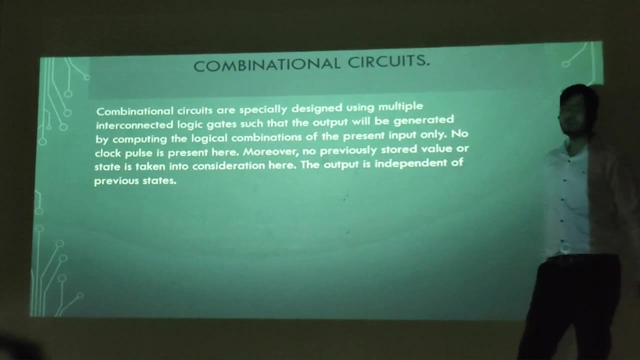 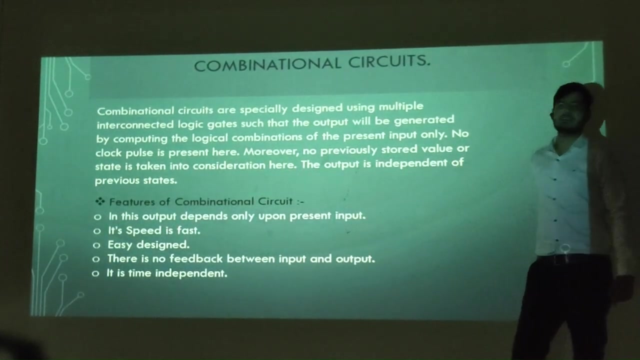 Combinational circuits are specially designed, using multiple interconnected circuits, Such that the output will be generated by computing the logical combinations of the present input only, And it is also the combinations of the logic gates, And the output is independent of previous circuits. So features of combinational circuits: 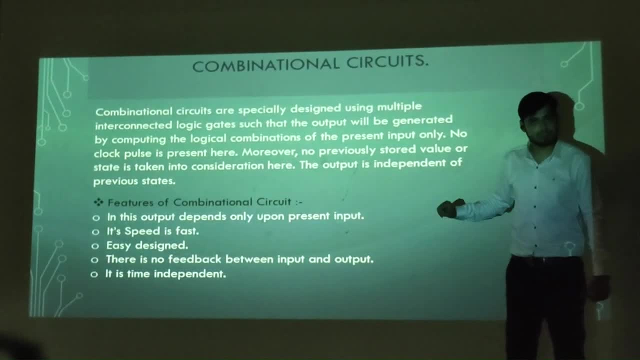 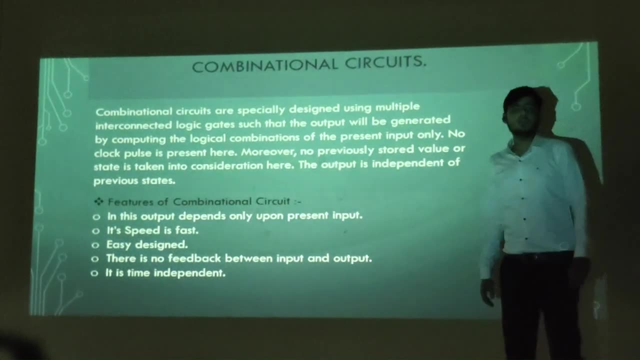 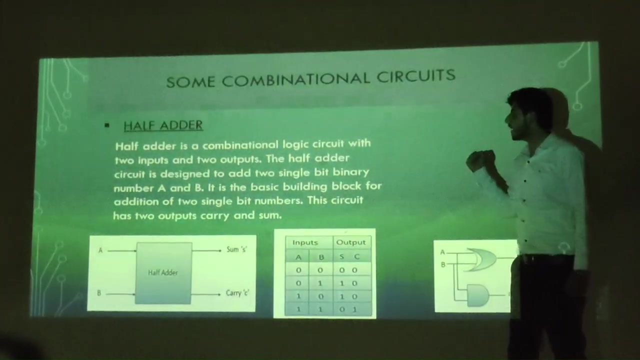 In this output depends only upon present inputs, Its speed is fast, easy design and its time is independent. So So Next we have to discuss some combinational circuits, In which first is half-address, Half-address is a combinational allergic circuit with two inputs and two outputs. 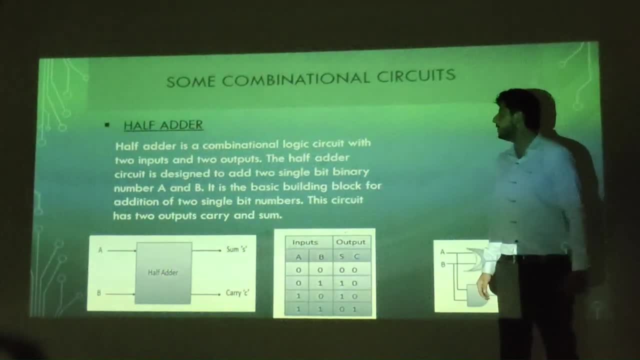 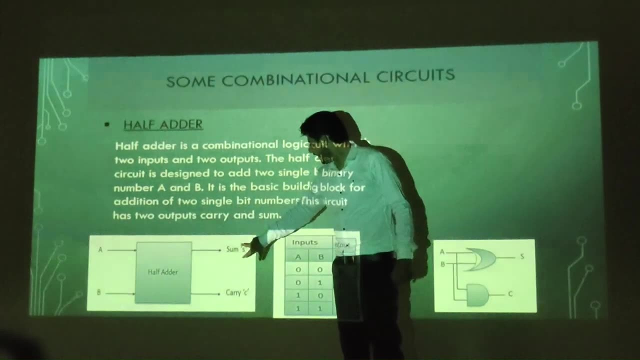 The half-address circuit is designed to add to signal hit by a number- A and B. As you can see here, this is a diagram of half-address In which two inputs are there- A and B- and two outputs- Some has and carry C. 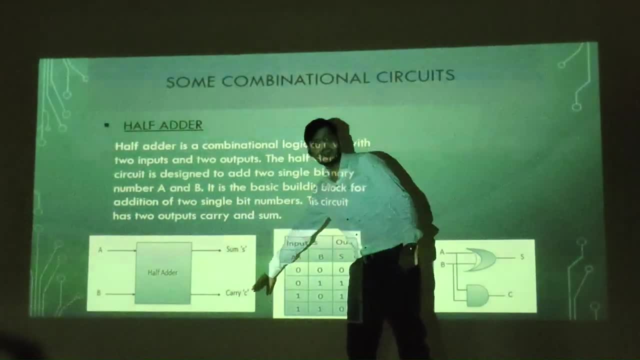 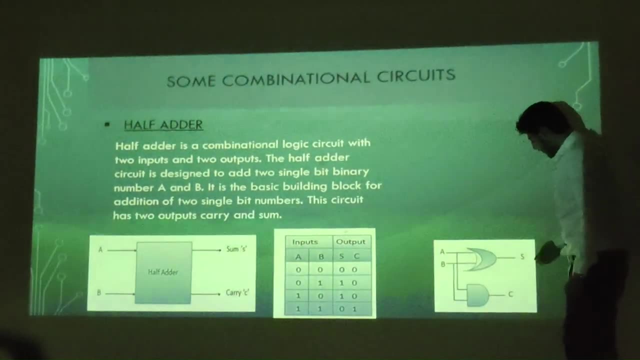 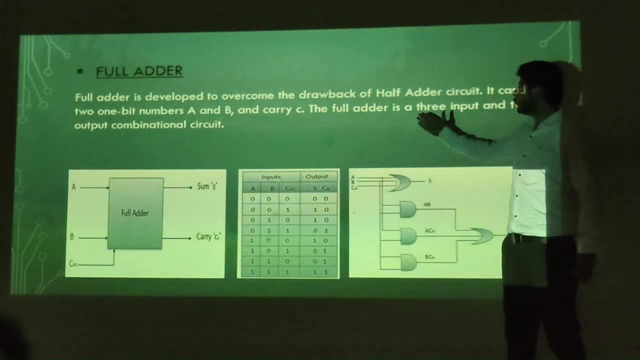 Which firstly, do the sum of the inputs and carry, gives the return scale. And this is the table. As you can see here. it is the Boolean diagram of cloud. Next is full header. Full header is developed to overcome the drawbacks of half header circuit. 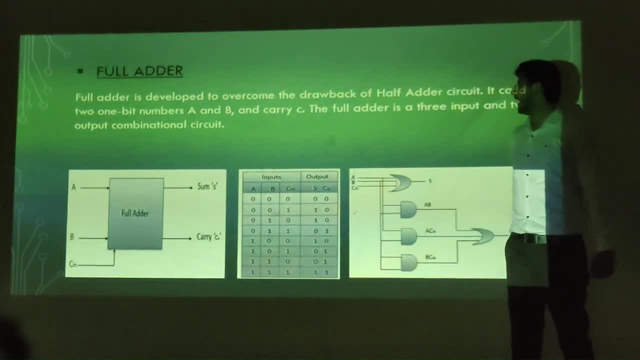 It can be 2 bit, 1 bit number A and B and N? C. The full header is a 3 input and 2 output combination of circuits. As you can see here, this is diagram of full header which has 3 inputs, 2 are A and B and